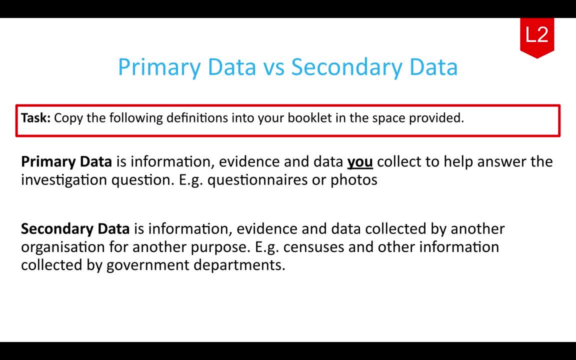 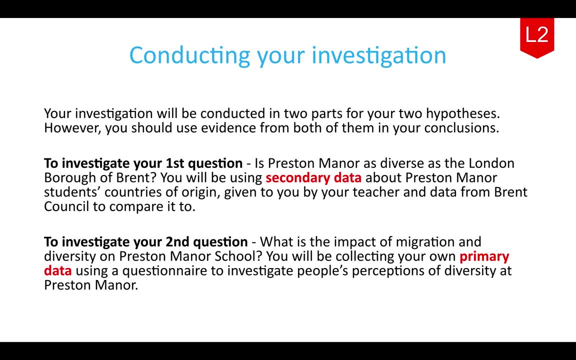 As you continue with this PowerPoint on your own, I want you to make your best effort to complete it. before you actually look at the answers, Try and work out what you think they will be Okay Now. the reason that all of this is so important is the following: There are two parts of our 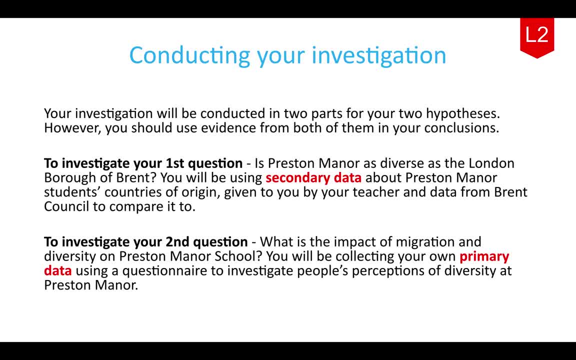 investigation. There are two questions and you picked your hypothesis last lesson. Today we're thinking about our first investigation question. Is Preston Manor as diverse as this London bar of Brent? And in order to do that, we can't really collect our own data. 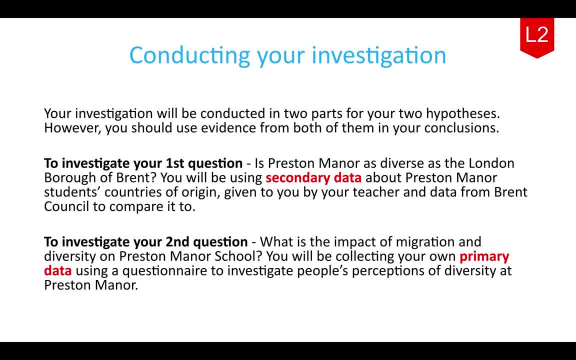 We can't speak to every single person in Brent and find out where they're from, whether they're as diverse as Preston Manor is, So we're going to have to use some secondary data. We're going to use data that the census gives us, that Brent uses. We're going to have to use some secondary data. 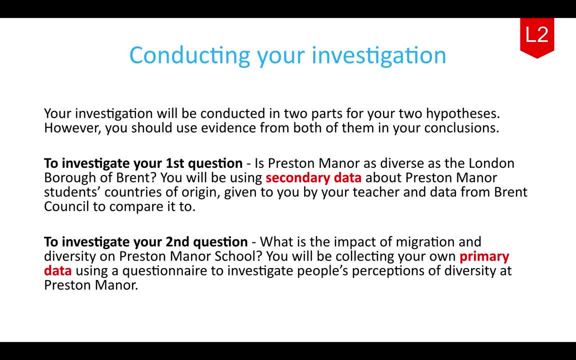 We're going to use data that Brent gives us And we're going to use data that I've taken off our school systems to see who is in our school and whether those two pieces of secondary data can be compared. So we're going to be looking at Preston Student Manor's students at Preston. 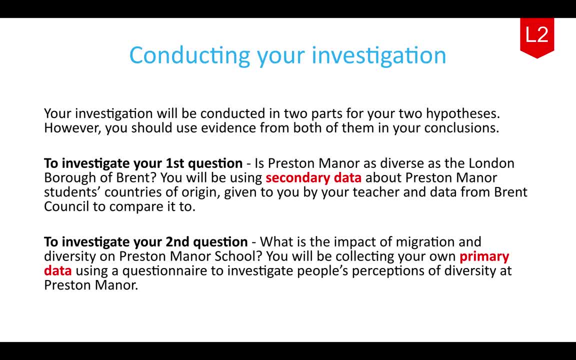 Manor's country of origin, which I'm giving to you, And we can look at data from Brent Council to compare it to. Okay. For the second question, though, it's a very different one. It's a very much more subjective and opinion-based question. Here we're asking: what is the impact of migration? 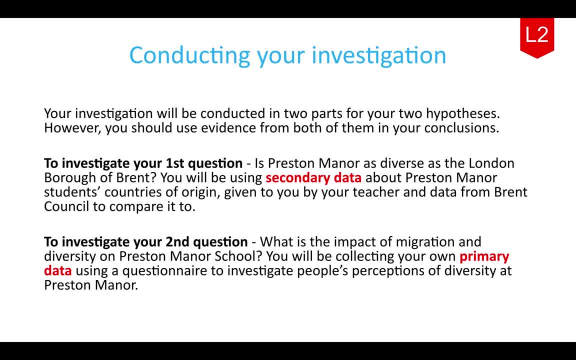 and diversity on Preston Manor school. We know that we're diverse, but what does that mean for us in our daily lives? So you're going to collect your own primary data, using a questionnaire, to see what people's perceptions of diversity at Preston Manor are like. We want to know what. 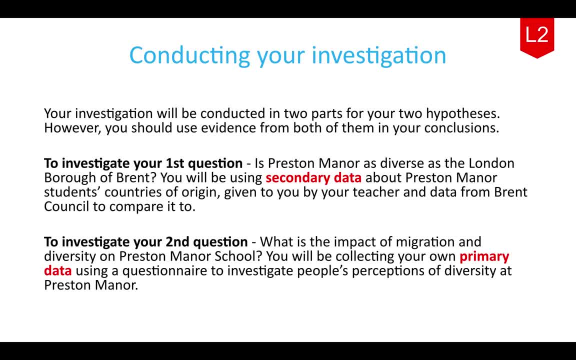 people think about the diversity. Is it a good thing? Is it a bad thing? In what ways That is going to require you to send your Google forms, to use your Instagram followers or your Snapchat followers to get them to start thinking about what they?